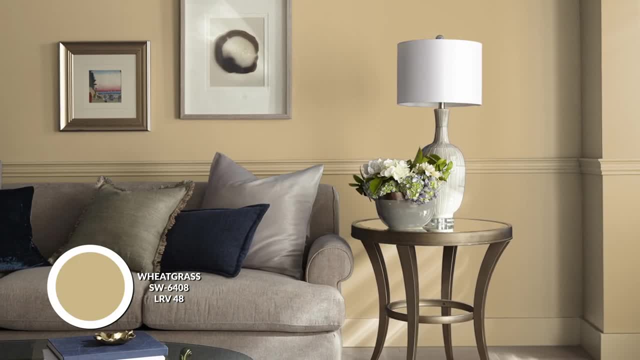 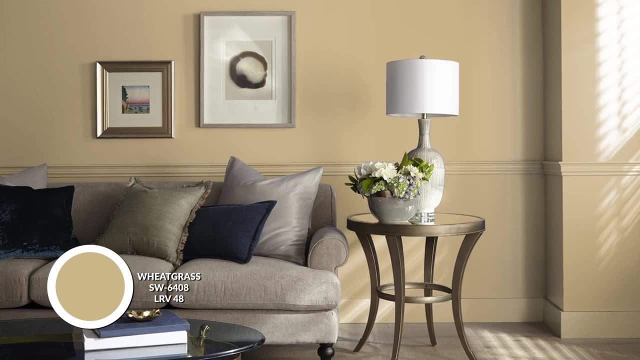 even though it has a green undertone, It's not a yellowy green by any means. So this is a great secondary color If you want something a little more saturated and deep. also just an interesting mid-tone neutral choice. The third color is a semi accent. It's very different from the other two. 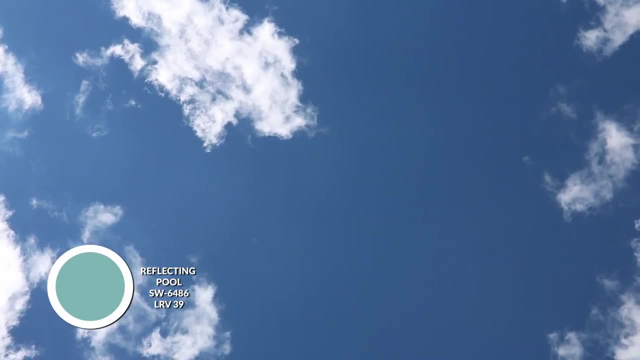 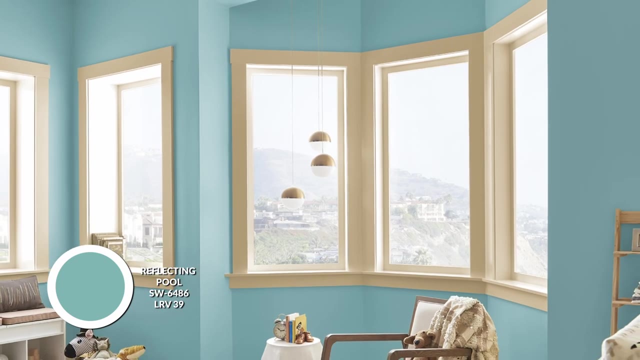 It's called Reflecting Pool And this color has a bit of a sky blue feeling to it. It is a little more on the warmer side, though. It has a slight yellow undertone, so not quite a greeny blue, but definitely on that side of things rather than a true blue or 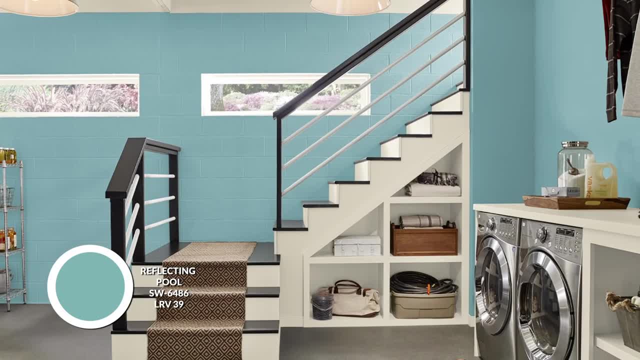 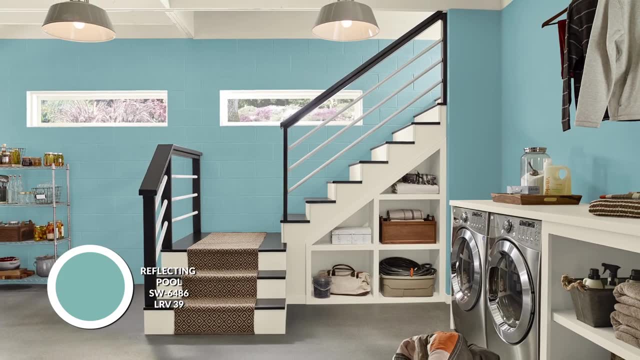 even an indigo type of coloration So it will help pick up on the yellows in the other colors, but very much a blue, So you will have a beautiful, fresh, airy sort of feeling to it. It is darker. It has a 39 LRV so it's technically the darkest color so far. 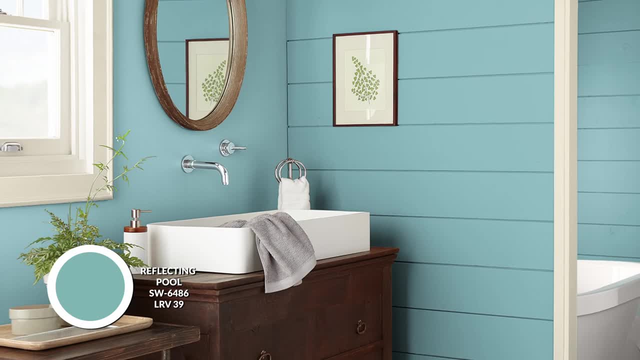 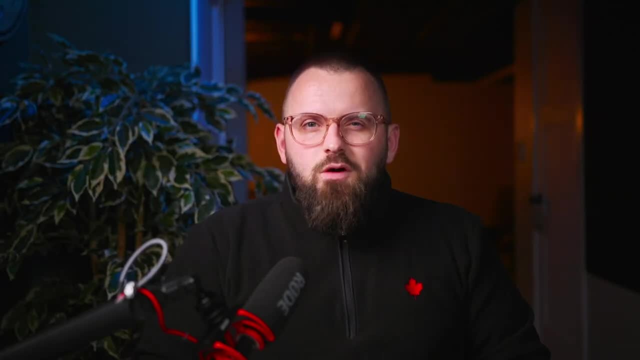 but a great choice in those sectioned off areas of your home, like bathrooms. for sure, Even if you're in bedrooms can be a good choice, but you can also use this in a living room if you want something that's very different and fresh and uplifting. Now for our fourth color. you may have noticed 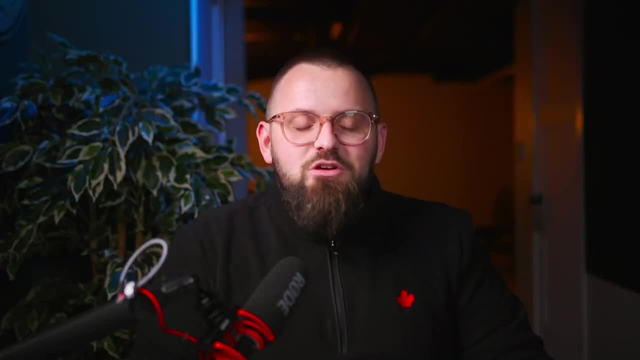 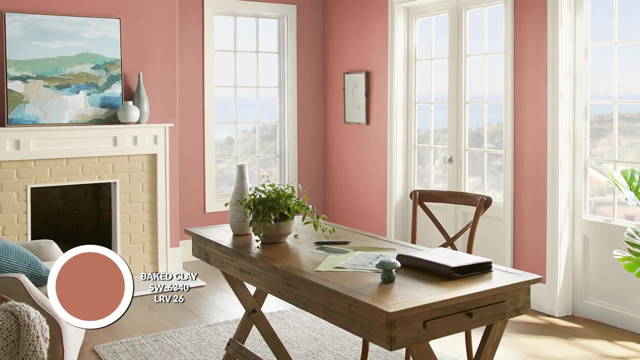 we're getting darker and darker and darker and the trend continues with Baked Clay. This is actually an expert pick, Sherwin-Williams color. Take what you will from that. but it also leans into that red undertone that is very prevalent in today's design. Red and point is the color. 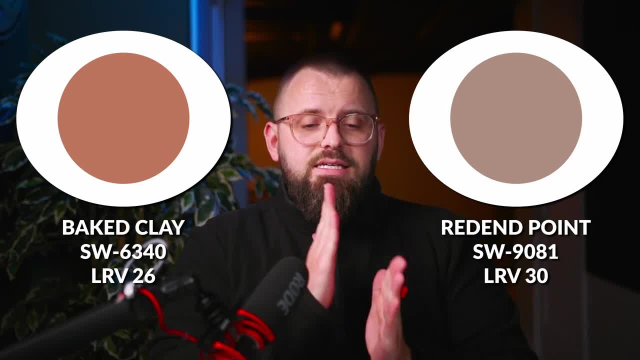 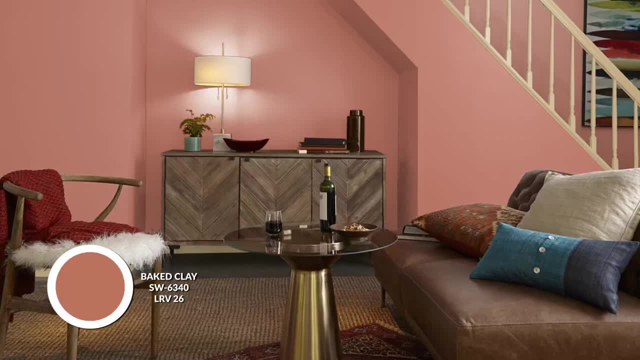 of the year currently for Sherwin-Williams, Baked Clay is cut from the same cloth. It has that red clay feeling which there is a ton of in the Southwest, And I think this is a color that could traditionally be seen as an accent color because of how saturated and dynamic it is. 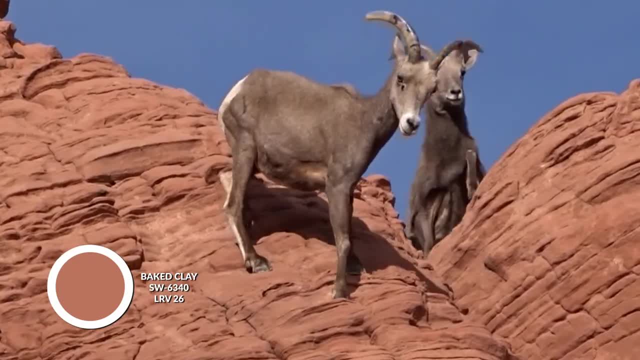 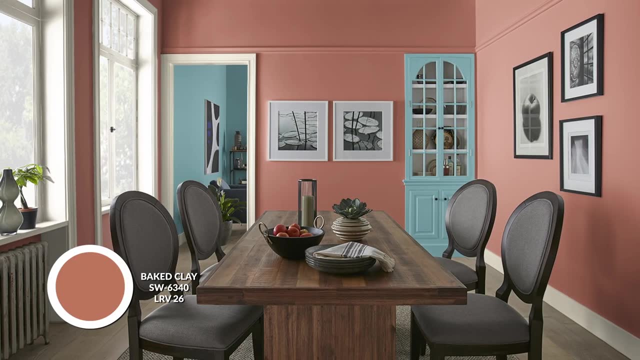 but it's also earthy. It's also totally appropriate for that part of the United States. So it's a color that you can use as a secondary color, not just in an accent wall format, but you can have your dining room this color, even a kitchen maybe, if you wanted. It is an. 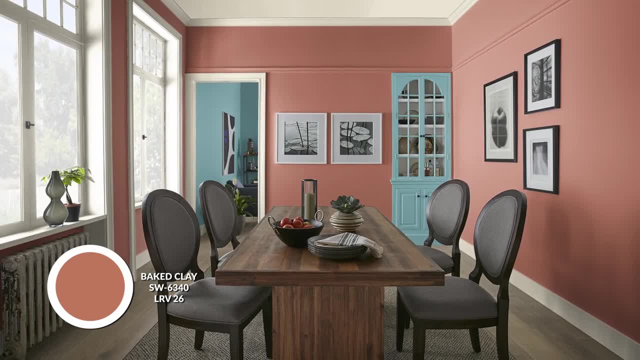 interesting one to me because it has that dusty quality to it That does make it a little more versatile than just a straight up red. So I'm going to go ahead and start with Baked Clay. I'm going to go ahead and start with Baked Clay. I'm going to go ahead and start with a bright.